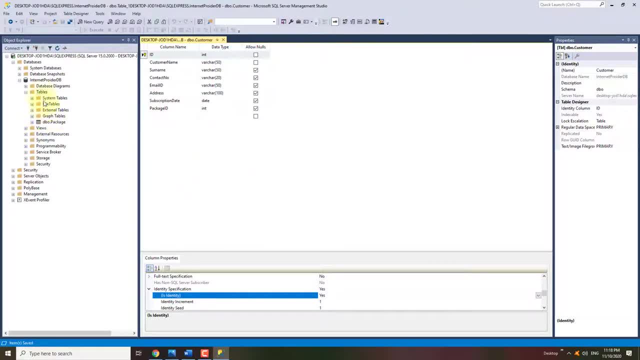 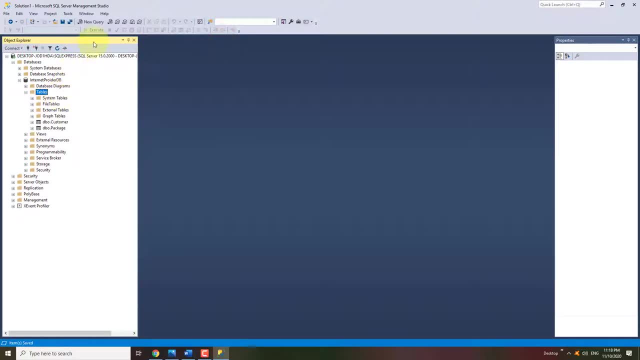 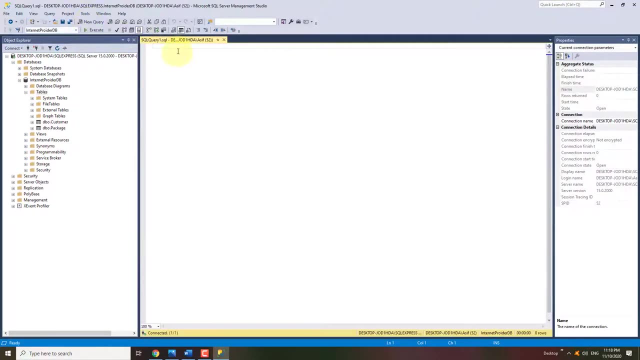 You can also create tables using the SQL query window. Let's build the third table using SQL query window. Keep the tables folder selected. Click on the new query option in the top menu options bar. Write the create table SQL query. Click on the parse option to check for syntax errors. 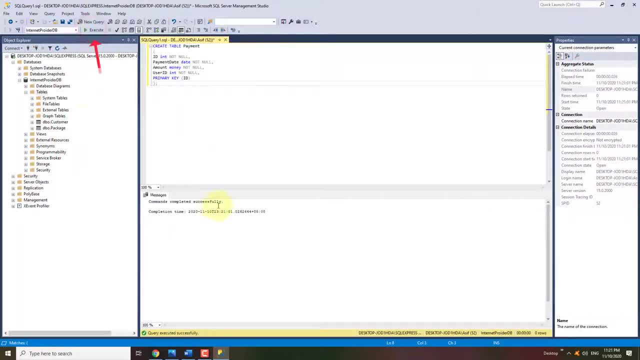 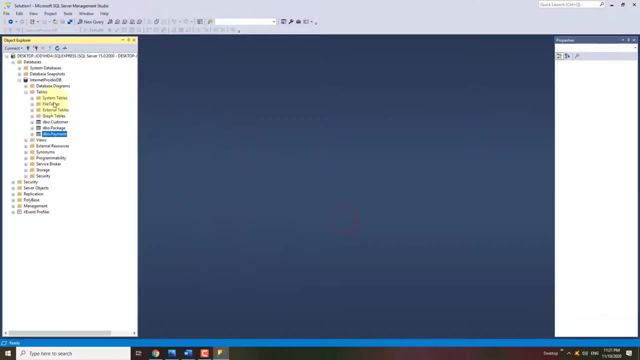 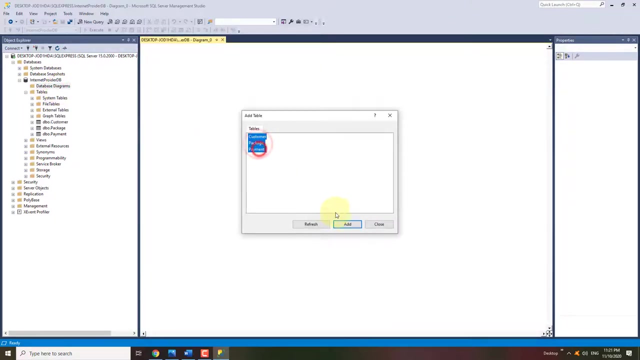 After that, click on the execute option to execute the SQL query. Refresh the tables folder and the table is successfully added to the tables folder. Now let's create the relationships model using SQL Server. Expand the database diagram folder. Install any missing modules by clicking on the yes option. 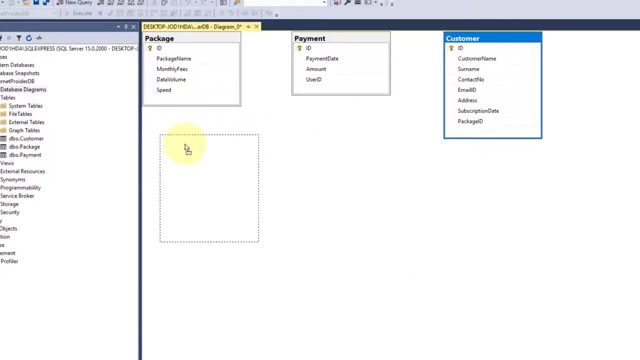 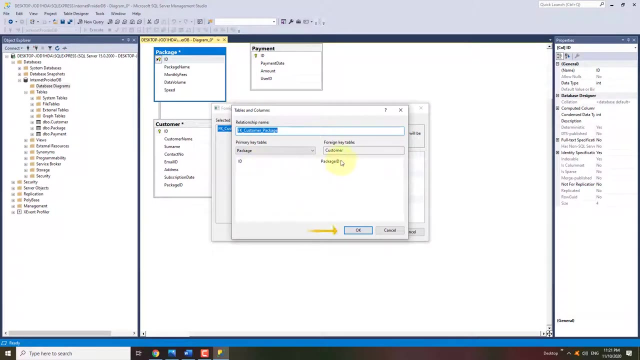 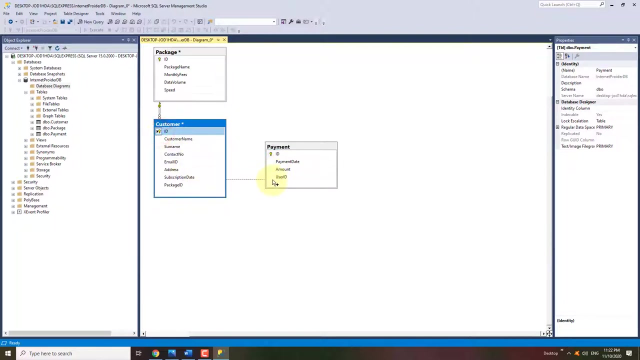 Arrange the tables by dragging the tables to the appropriate positions. Click on the primary key of the first table And then click on the table where you want to use it as a reference. Choose it as a reference key. Similarly, make the relationship between the second and third table. 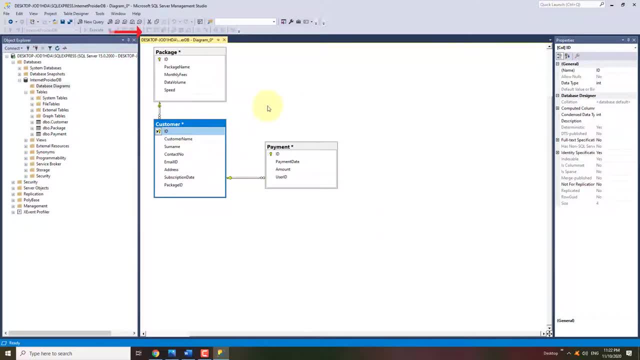 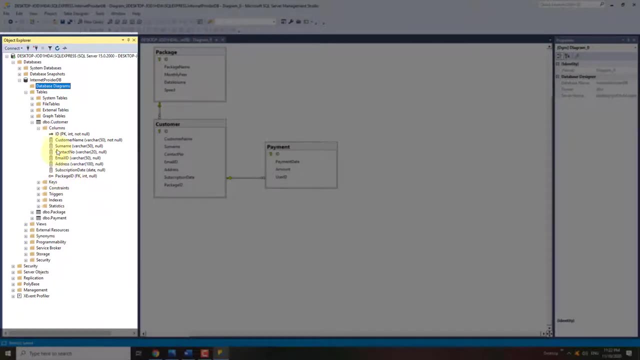 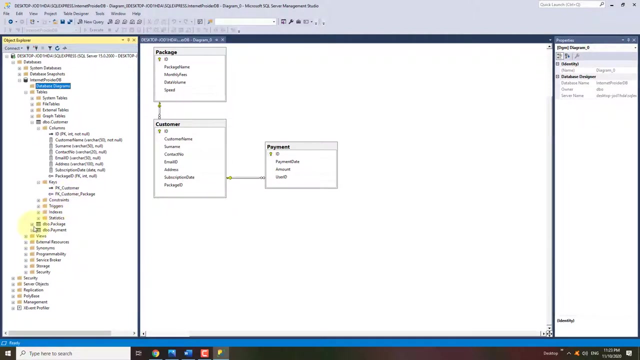 Right click on the diagrams window and select save diagram. Press Ctrl plus S keys, Name the diagram and press enter. The relationship table is created successfully. Now you can check the primary key and foreign keys for each table in the tables folder. Right click on one table and click on added top 200 rows. 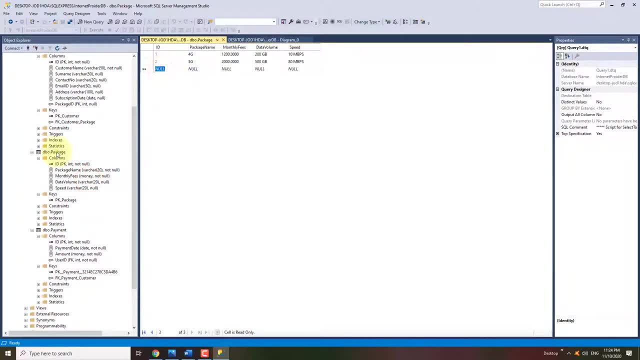 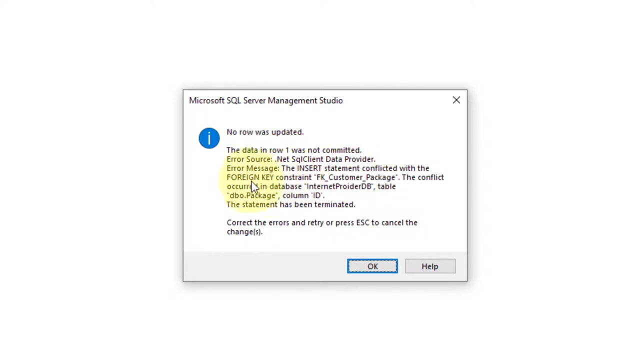 Add records to the first table. Now again right click on the second table and select added top 200 rows. Enter any record in the child table. The child table's foreign key column gives an error because package ID 4 is not present in the parent table.